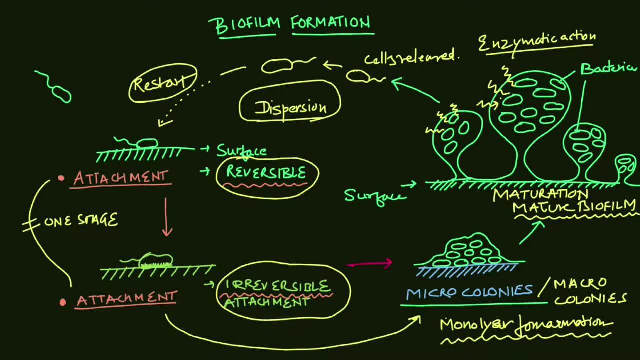 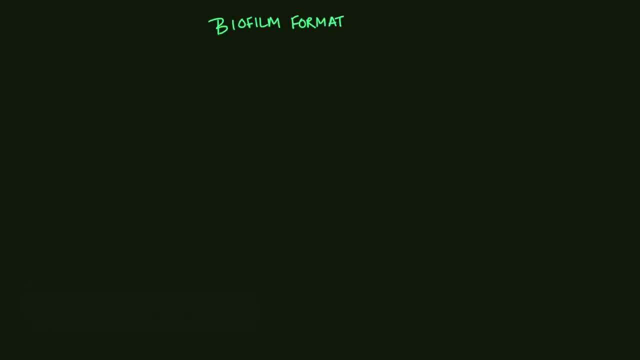 I hope this video is going to help you to understand the process of biofilm formation. Let's start the discussion of biofilm formation. in the first stage, what will happen? the bacterial cell will try to attach to a solid surface and that stage is the attachment stage. so here you're seeing: bacteria is getting attached to the surface. 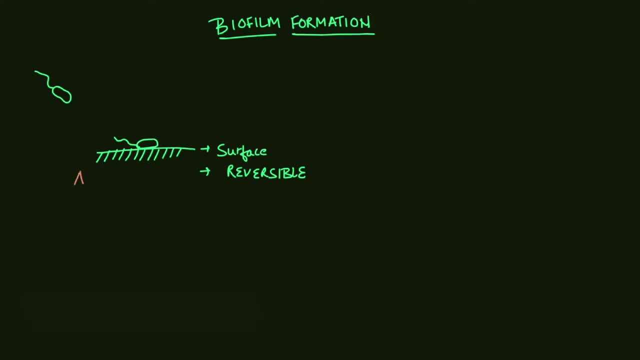 and the attachment is reversible in this case. initially it is reversible. so this i can say: it is the first stage, which is the attachment, and the stage where you have cells reversibly attached to the surface. and then you have second stage where the cell will firmly, or i would say well tightly, attached to the surface. and this stage 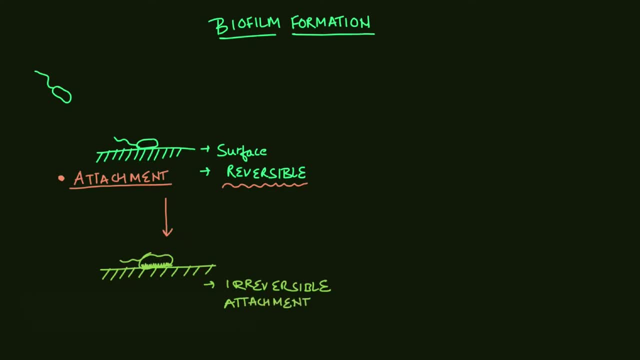 is the irreversible stage where cell no longer able to detach from the surface. and this is the again, this is the part of the attachment stage. so you have two different stages in the attachment stage, two different sub stages. next you will have the formation of monolayer, or it's also known as micro colony formation, and then they will develop into 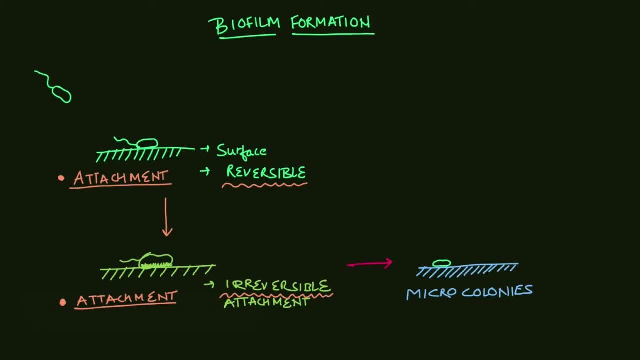 macro colonies. so it will be micro as well as the macro colony formation where cells will divide and then they will constitute the colonies on that solid surface. after that you will have the dispersion, where three-dimensional colonies. they will appear on the surface and, as you can see, 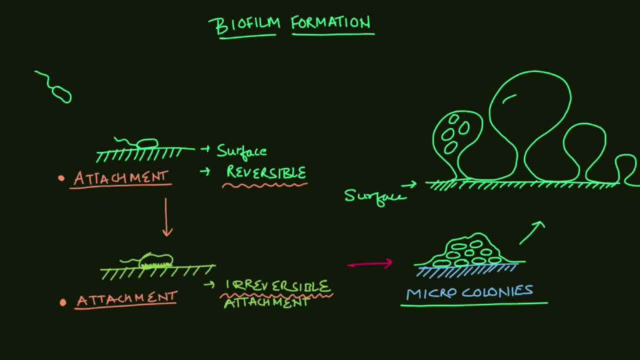 here. cells are inside these three-dimensional colonies and they will constitute a mature biofilm. so this stage is called as the maturation stage. after that you will have the stage of dispersion, where the cells they will detach and then they will again start the process of attachment and form the new biofilm. so as 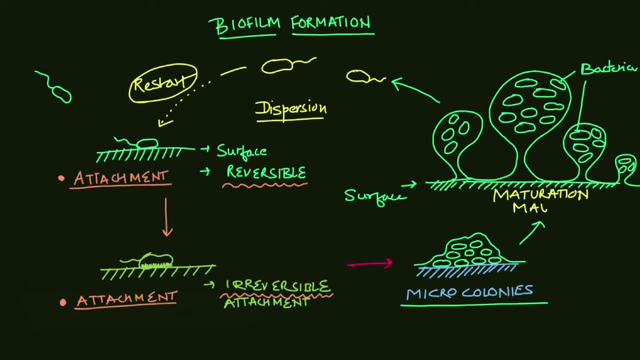 you can see here, this stage is the maturation, or it's also known as mature biofilm, and stage that is previous to that, that is, the micro or the macro colony formation. so you have different, different stages. that includes the formation of biofilm by, specifically by, bacterial cell. let's